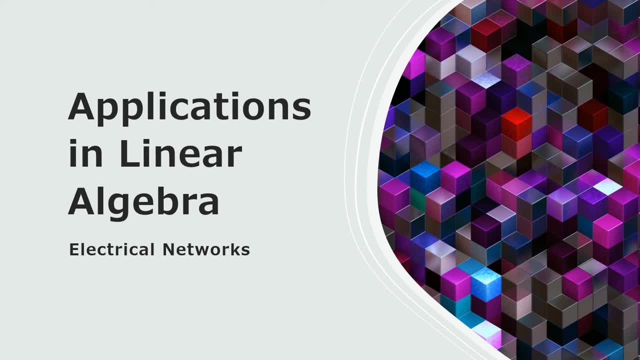 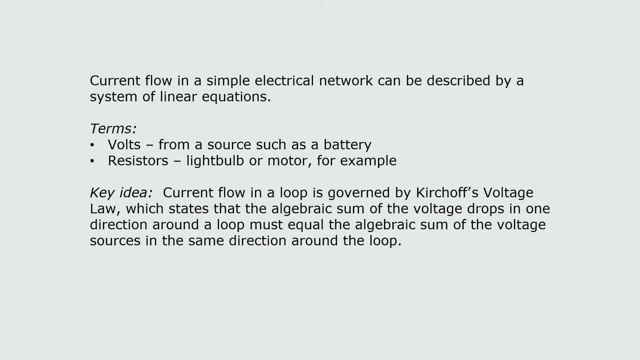 In this video we're going to look at an application of linear algebra and we are going to look at electrical networks. So here's the idea with electrical networks. The current flow in a simple electrical network can be described by a system of linear equations. There are some terms that you need to know. 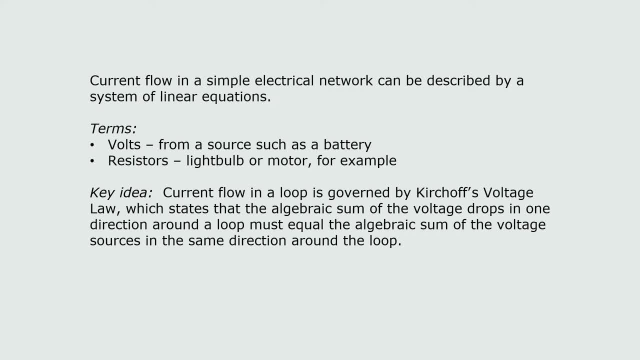 Volts is from a source such as a battery, and resistors are things such as light bulbs or motors, for example, that use up the power. The key idea when you're setting up your system of equations is that current flow in a loop is governed by Kirchhoff's voltage law, which states that the 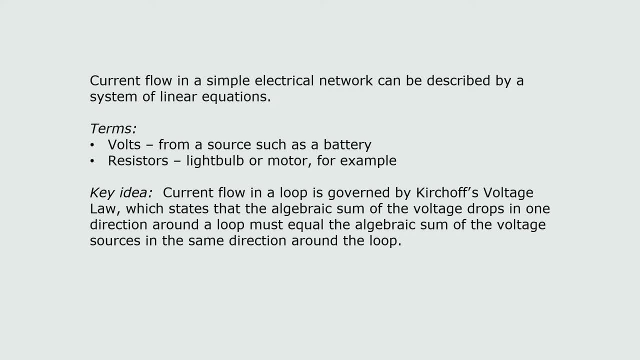 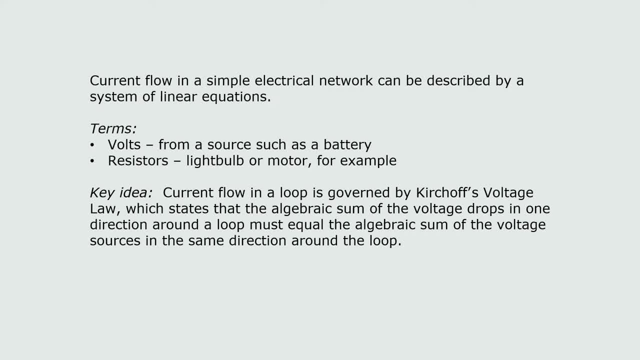 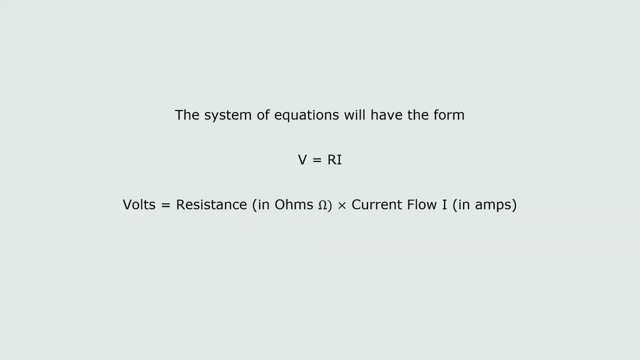 sources in the same direction around the loop. So in other words, we're not gaining or losing power in our loop. The system of equations is going to have the form: volts equals resistance in ohms times, current flow, which we use a capital I to represent in amps, So resistance is in ohms. 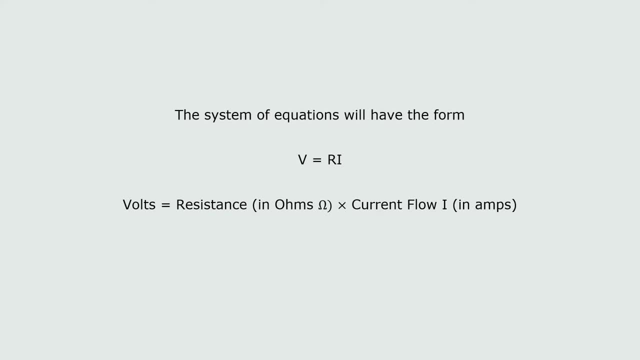 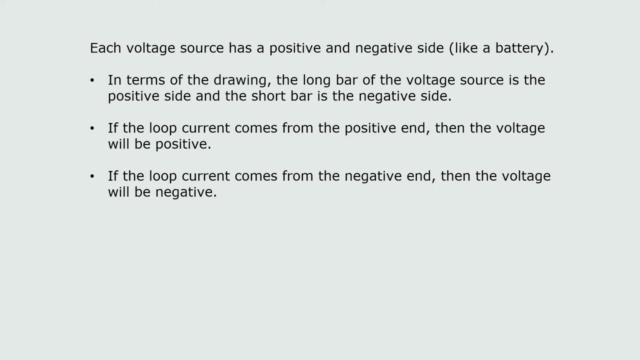 current flow is in amps and volts is itself in volts. So remember this form of the equation, because that's what we'll use to set up a matrix equation. Now, each voltage source has a positive and a negative side, like a battery does In terms of the drawing. the long bar of the voltage source is the positive side. the negative side is the negative side. 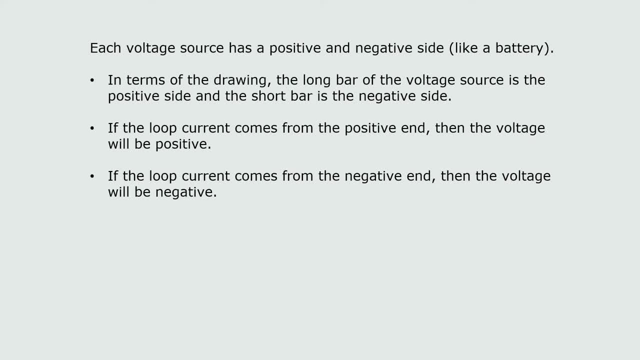 In terms of the drawing. the long bar of the voltage source is the positive side, the negative side is the negative side And the short bar is the negative side. If the loop current comes from the positive end, then the voltage will be positive, and if the loop current comes from the negative end, 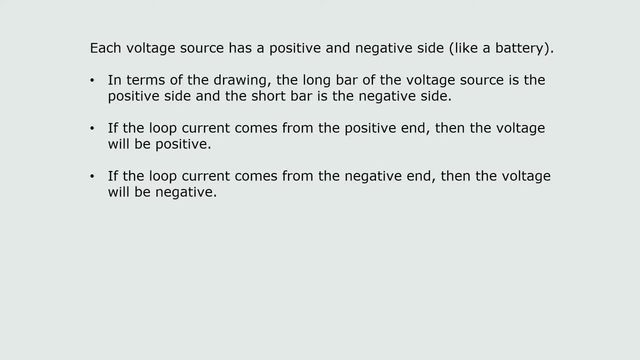 then the voltage will be negative. So let's see how this would actually look. So we have a battery and it's drawn with a long edge and a short edge. Now we have a loop current coming from either the long side or the short side, and in this one I just drew 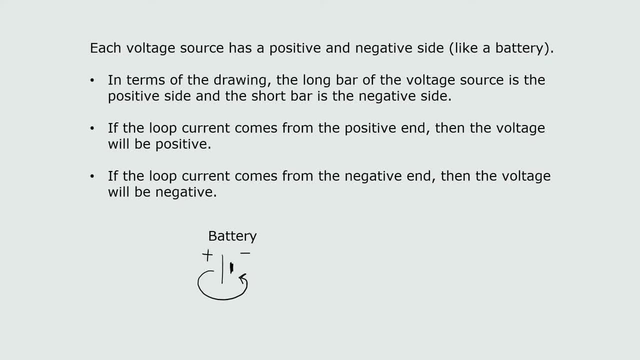 the loop current is coming from the long side of the battery, which is the positive side, and so my voltage is going to be positive. Alternatively say, I had my battery and the loop current is coming from the short end or the negative side. In that case my voltage is going to be negative. So you will need to know that. 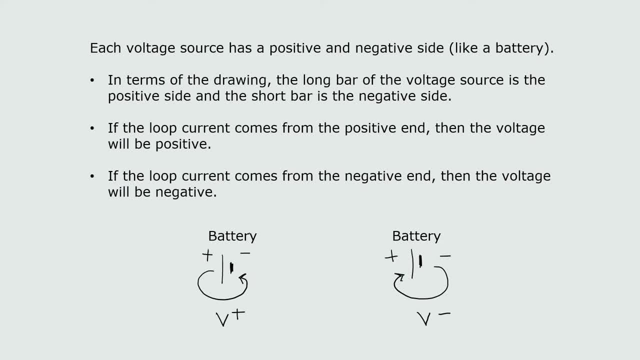 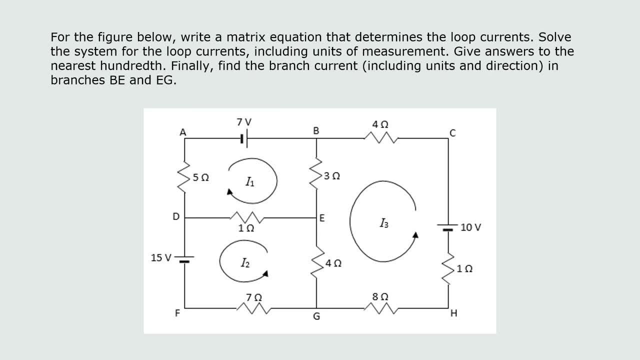 the voltage is coming from the negative end and that the voltage is coming from the short end. So you can just look at the picture that you're trying to set up a matrix equation for. Okay, so here's the example we're going to work through For the figure below. write a matrix: 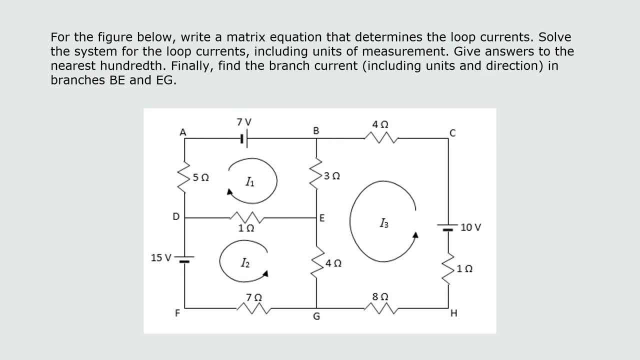 equation that determines the loop currents, Solve the system for the loop currents, including units of measurement, Give answers to the nearest hundredths, so two decimal places, And also give an answer for the number of units, including units and direction in branches, be and eg. 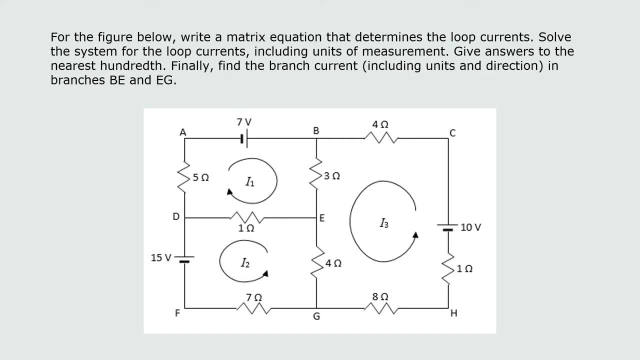 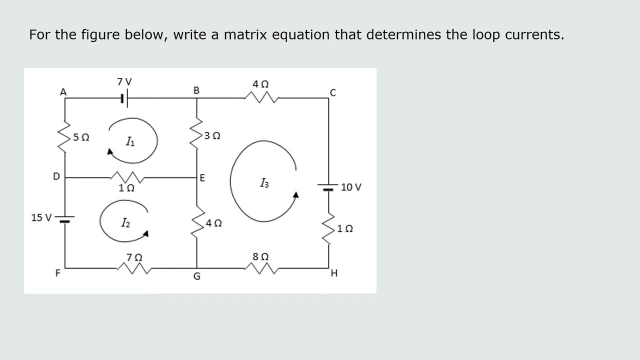 So this is really asking us to do three things. So let's just focus on the first one. The first one says: for the figure below, write a matrix equation that determines the loop currents. So we're given a picture of what our electrical network looks like. 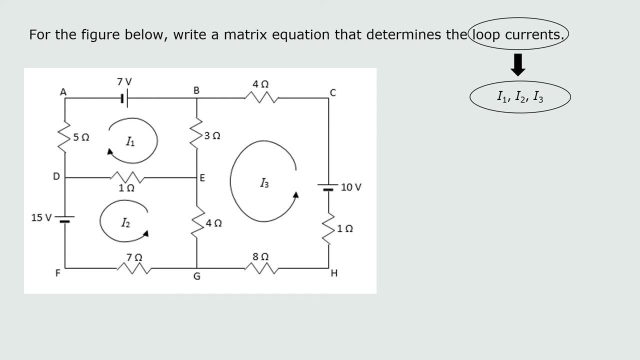 What we're going to do is we are going to find the loop currents, which are the I's. Remember currents are in amps and they are represented by a capital I, So loop currents are the I1,, I2, and I3.. 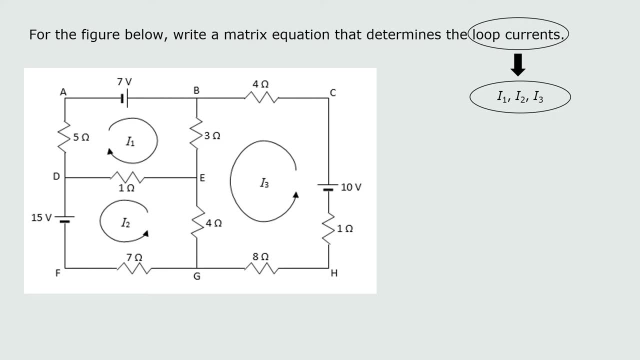 If you had a larger system you could have more than three loop currents, But in this picture we only have three. Now remember the relationship that voltage equals resistance times, current flow, And the current flow is the I, the I1,, I2, I3. 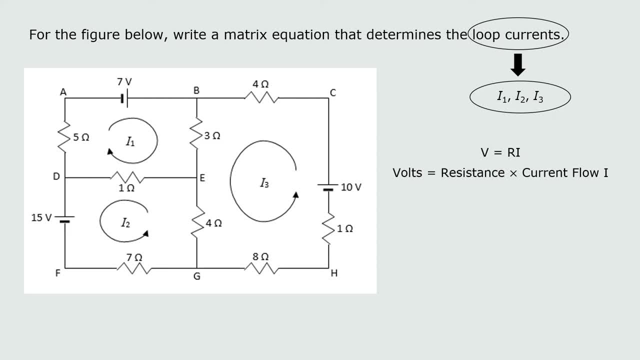 And volts is coming from the batteries, And then the resistance comes from these squiggles in our lines. Those are the resistors. Because we have this form of the equation. if we wanted to set up our system, I would probably reverse it and say that resistance times current flow equals voltage. 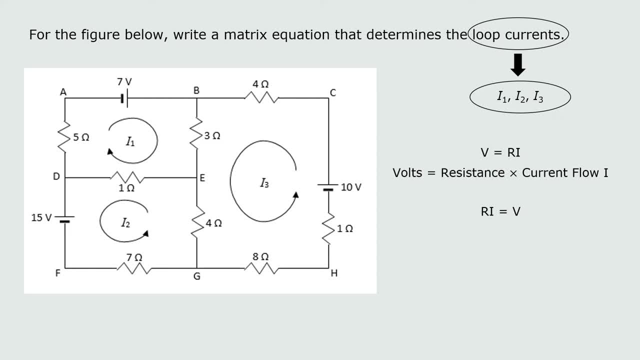 Because that's how we're used to seeing our system of equations set up, Where there's a matrix times a vector on the left side equaling a vector on the right side of the equation. So the form is going to look like this: I'm going to have a matrix that is made up of the resistors. 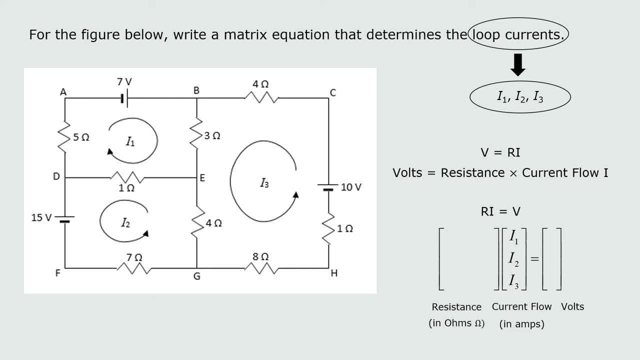 So I'll have resistance in O, Which is represented by omega times, the current flow in amps, And because we have three loop currents, that's going to be a vector with I1, I2, and I3 equals a vector that's made up of the voltages. 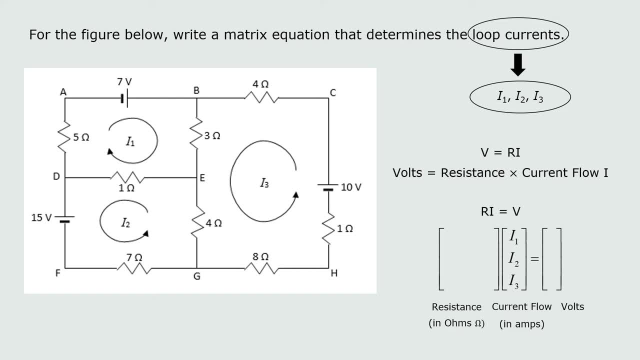 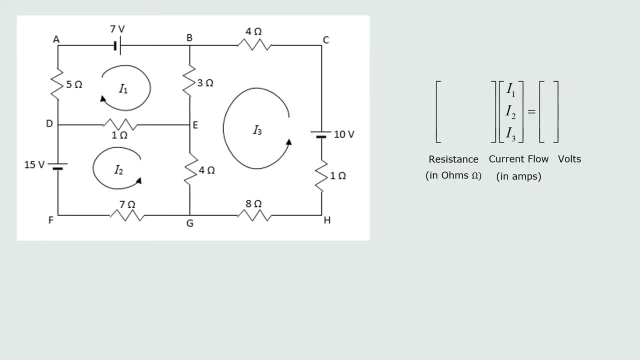 So what we want to do is figure out what goes into that matrix and what goes into the voltage vector. Okay, so here's what we have, And what we want to do is break it down by loop. So I'm going to look at loop one, loop two and loop three separately. 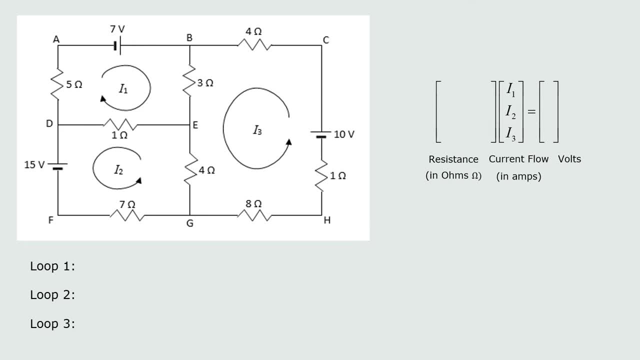 So we'll start with loop one, And what we look at is we look at the current flow to start with. So I see that that current flow is going clockwise, And so that means that I'm going to view this loop, loop one- clockwise. 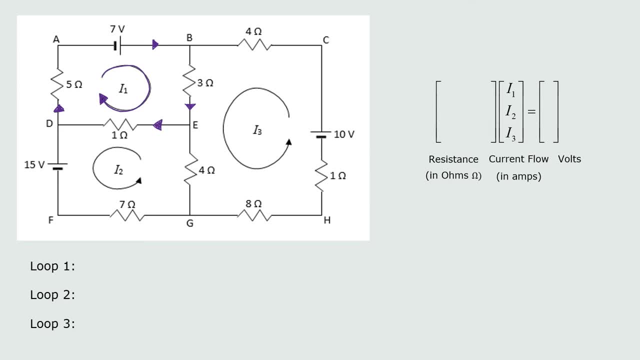 Okay, So I look at my resistors. When I1, the current flow goes through this loop, It goes through three resistors. It goes through the three ohms resistor, the one ohm resistor and the five ohms resistor. 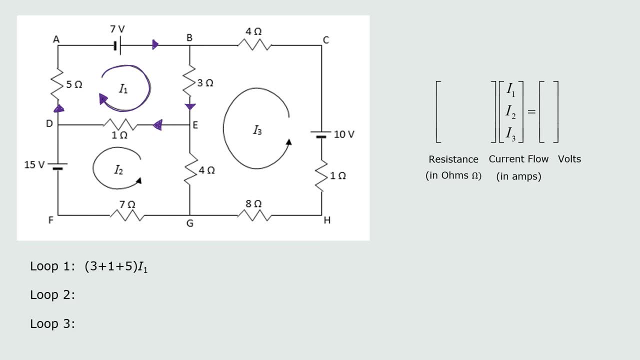 So for I1, the resistance is three plus one plus five. So that's my resistance times current flow. Okay, So three plus one plus five, I1.. Now still within loop one. I want to see if any of the other currents go through loop. 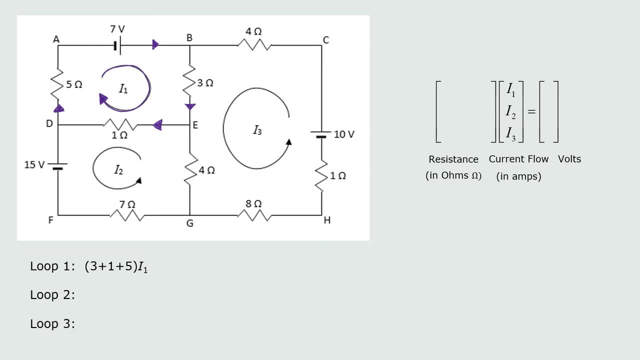 one. So if I look at the I2 current flow, I see that I2 is going counterclockwise And so when it goes through that one ohm resistor That is part of loop one, it is going the same direction as the I1 current flow. 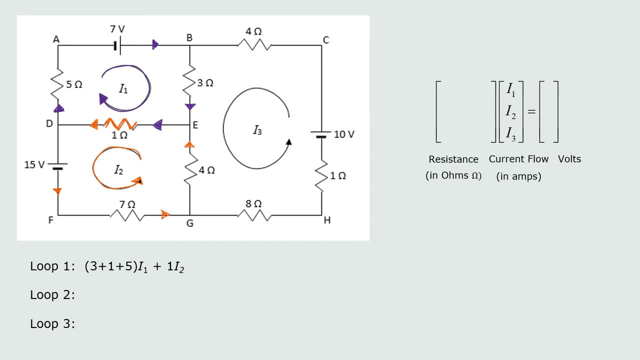 And so this is going to be a plus one I2.. So the resistance is one ohm and the current flow is I2 through that resistor. Now I look at whether or not I3 flows through loop one. So I see that I3 goes counterclockwise. 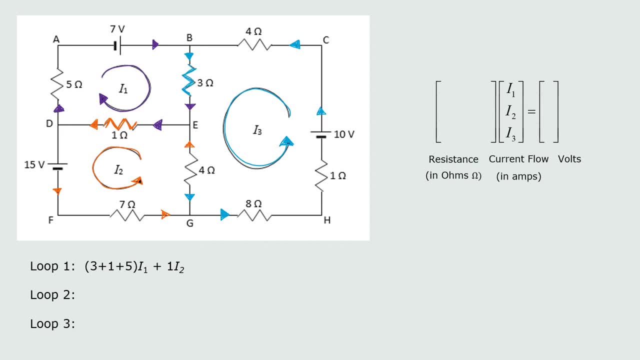 And it goes through the three ohms resistor of loop one. It's going the same direction as the current flow of I1. And so it will be a plus three times I3.. So the resistance is three. The current flow is I3. 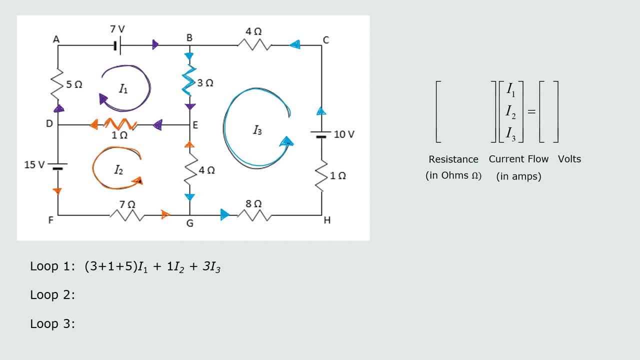 Now I have to figure out the voltage in loop one. So I look at the battery source or the power source And I want to figure out what the voltage is. So I look at the battery source or the power source And I want to figure out what the voltage is. 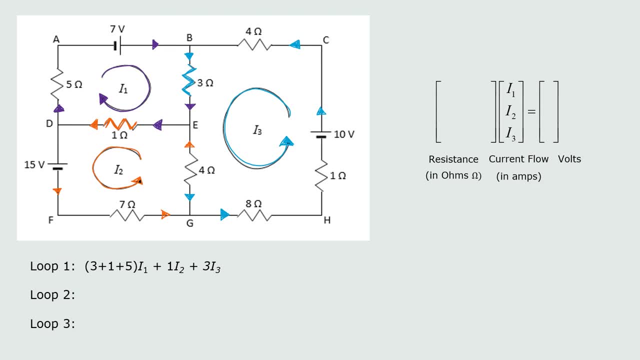 And I want to figure out whether my current flow is going in the positive or negative direction from that power source. And I want to figure out whether my current flow is going in the positive or negative direction from that power source. So remember, the long bar is positive, the short bar is negative. 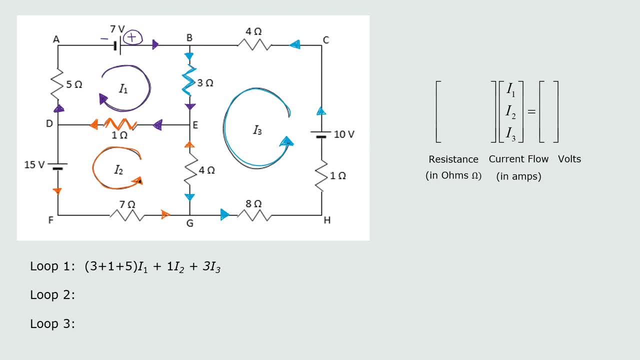 And my current flow is coming out of the positive end of the power source, And so this is going to be, for my voltage, a positive seven. so equals seven. So there's my loop one equation. Now I have to do the same thing for loops two and loop three. 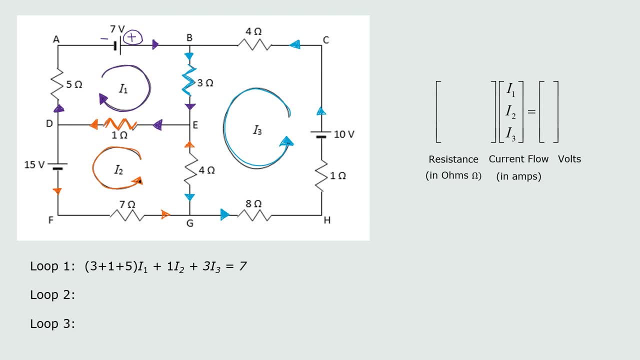 Now I have to do the same thing for loops two and loop three. So I already know in loop two that my current flow is going counterclockwise And I can see the resistors in loop two are seven ohms, four ohms and one ohm. 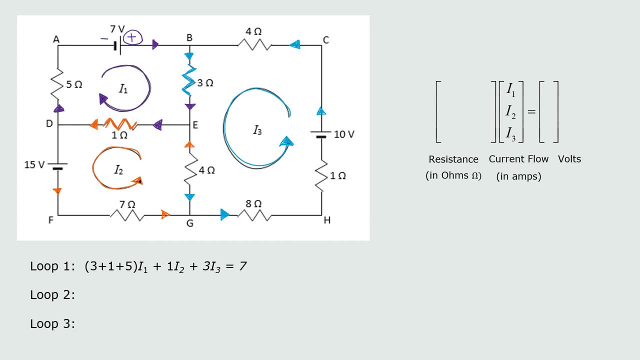 That one ohm resistor is part of both loop one and loop two. It's shared, shared between the two loops. So to get my I2 portion of loop 2, I'm going to add those resistors, 7 plus 4 plus 1 I2.. 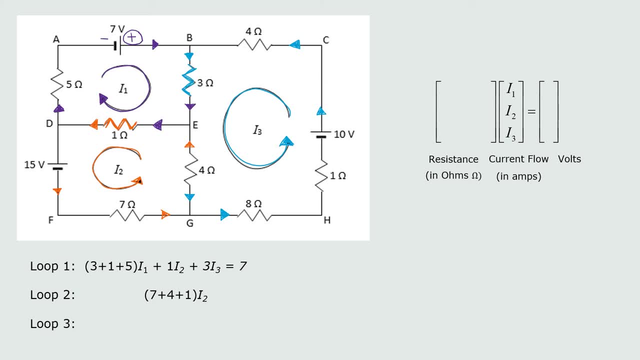 Now I need to look at what I1 is doing. Is I1 adding any current flow to loop 2?? Well, we already saw that loop 1 and loop 2 share that 1 ohm resistor and that the current flows go in the same direction through that resistor. 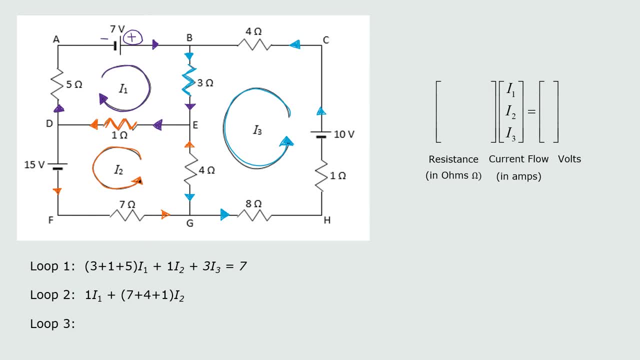 So I have a plus 1 I1. So I'm going to write that first I'm going to do 1 I1 plus the I2 portion, 7 plus 4 plus 1 I2.. Now I look at I3.. So I3 is going. 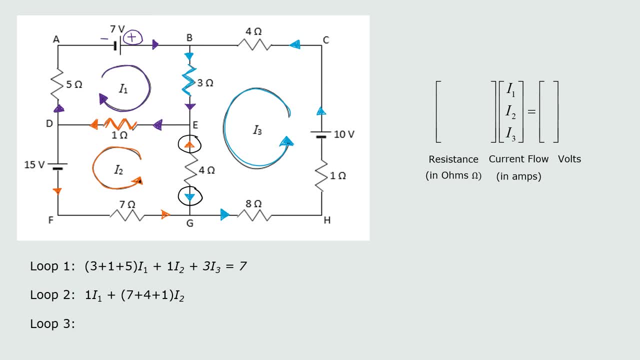 in the opposite direction from I2. And they are both going through that 4 ohms resistor, But I3 is going in the opposite direction, So it is working against I2.. And so this is going to be a minus 4 I3 in loop 2.. 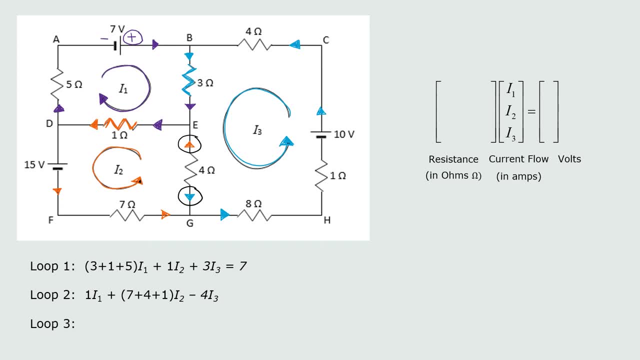 Now I look at the voltage. So the battery source or power source in loop 2 is the I2 current flow And the current flow is coming from the negative end of that power source. So the short end, the shorter, thicker bar. 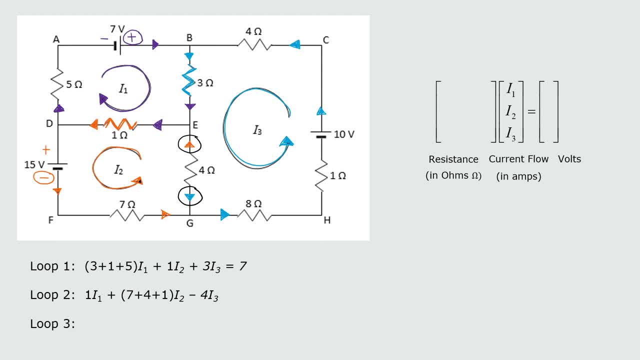 So my voltage is going to be a negative 15 for loop 2.. Now I move on to loop 3.. So loop 3 has several resistors. It has the 4 ohms at the top and then 3 ohms and 4 ohms on the left side. 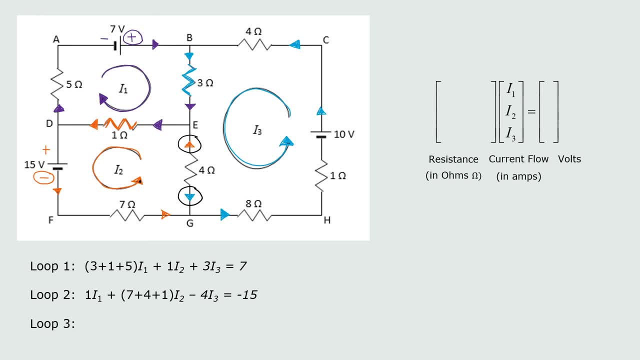 And then 3 ohms and 4 ohms on the right side, 8 ohms on the bottom and 1 ohm on the right side. So my I3 portion is going to be 4 plus 3 plus 4 plus 8 plus 1.. 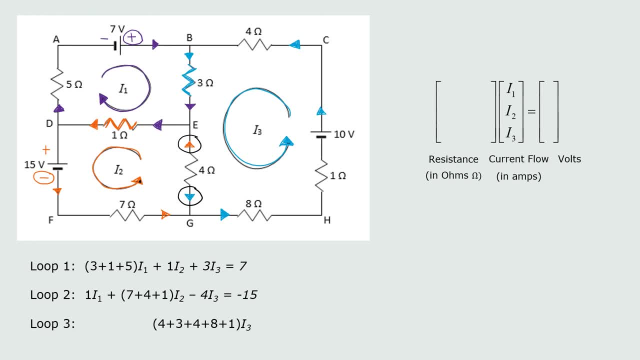 That is the resistance for the current flow I3.. Now we already know that loop 3 and loop 1 share the 3 ohms resistor, So I will have 3 I1.. And we know that loop 2 and loop 3 share the 4 ohms resistor, but in opposite directions. 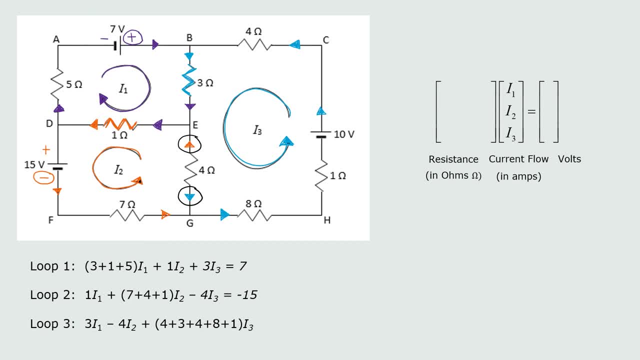 And so I will have a minus 4 I2.. For our power source, I can see that the current flow I3 comes out of the long side of the power source or the positive side, So I will have equals positive 10 for my voltage. 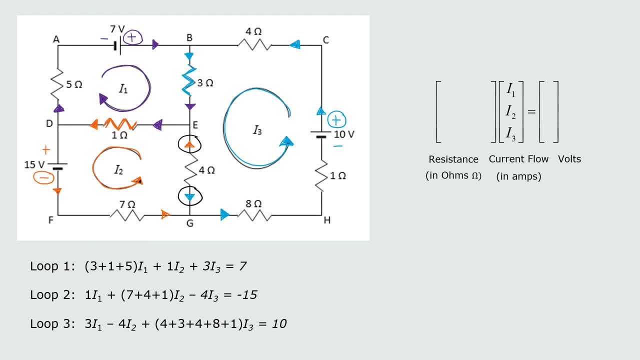 And now, basically, you have a system of equations with 3 equations and 3 unknowns, And we know how to put that into a matrix equation. So we are just going to put our coefficient matrix- 9, 1, 3, 1, 12, negative 4, 3, negative 4, 20. 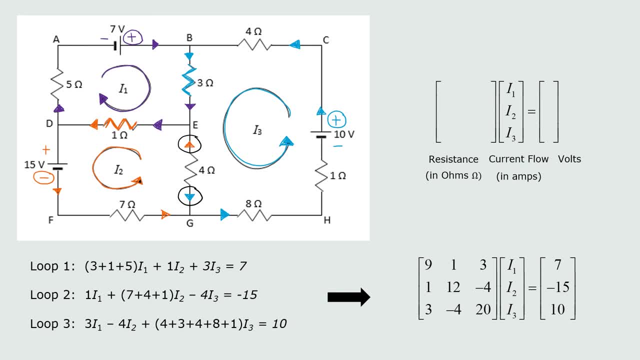 times the vector I1, I2, I3 equals our voltage 7, negative 15,, 10.. And this is what you will be asked to do in the case study- is set up your matrix equation. that would give you the answer. 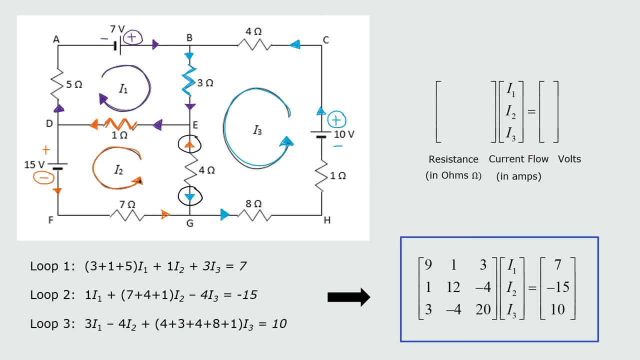 So that would be what you would answer in my labs for case study 1.. Okay, now this example problem that we are working through says to solve for the current flow. So what we are going to do, we are going to take that matrix equation. 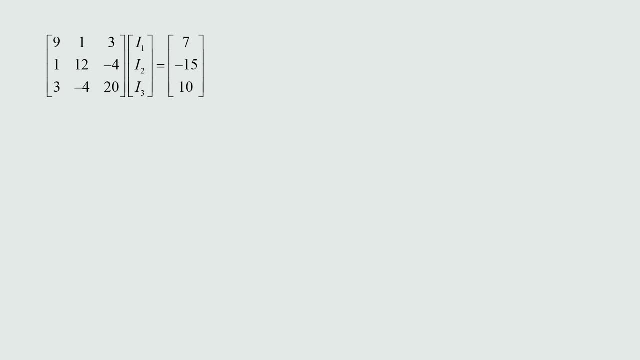 put it into an augmented matrix and find the reduced row echelon form. So I have done that here to solve for the loop currents. My reduced row echelon form is 100.88,, 010, negative 1.29, and 001.11.. 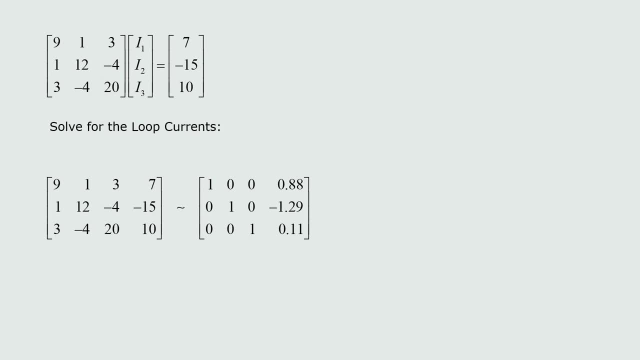 Now remember: each column of my resistance matrix represents a coefficient of I1,, I2, or I3. And the first column is I1,, second column is I2, third column is I3. So I have my solution here. I have a unique solution. 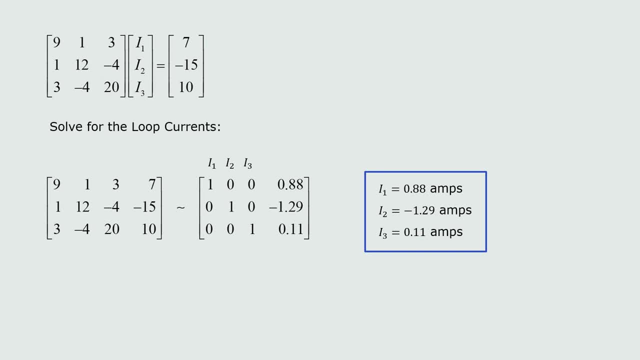 Current flow: I1 equals 0.88 amps, I2 is negative 1.29 amps And I3 is 0.11 amps. So that would be my solution for the current flow I1,, I2, and I3.. 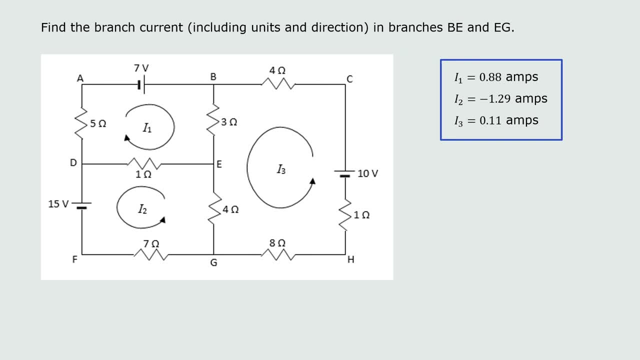 Now I'm asked to find the branch current, including units and direction, in branches BE and EG. So I'm going to do these separately. So BE, I'm going from B to E, And for branch BE, the currents that go through this branch, from vertex B to vertex E, are I1 and I3. 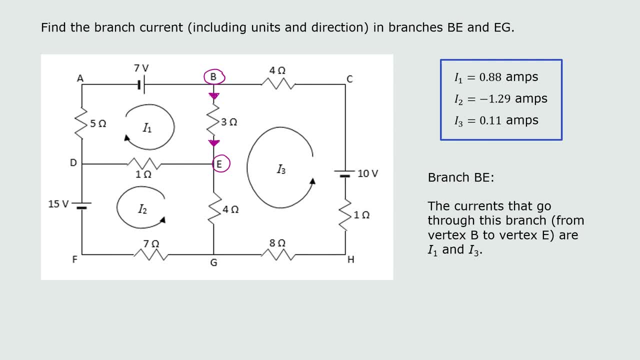 So what I'm going to do to find the branch current is add those two currents together. So the branch current in BE is I1 plus I3, which is 0.88 plus 0.11, giving me 0.99 amps in the direction of I1 and I3. 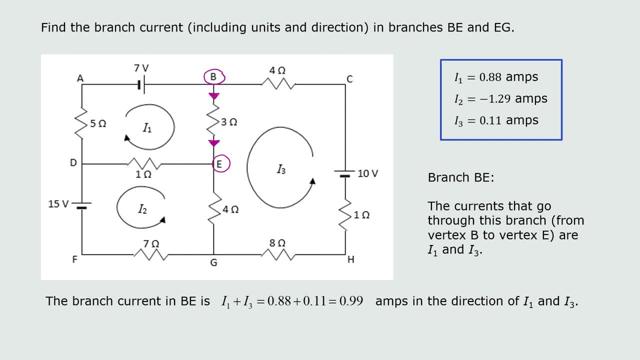 They're going the same direction, So I don't have to worry about which one it's going in the direction of, because they're both the same And they both are going from B to E. So that's why they are both positive in this sense. 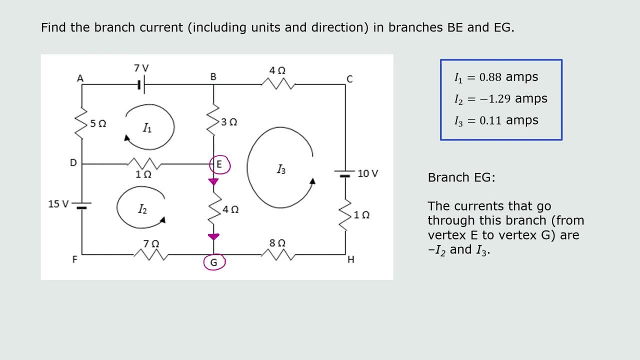 Okay, Now I'm going to find EG. So for branch EG, the currents that go through this branch from vertex E to vertex G are negative I2 and positive I3.. It's a negative I2 because it is going the opposite direction in the branch when I actually follow the current flow. 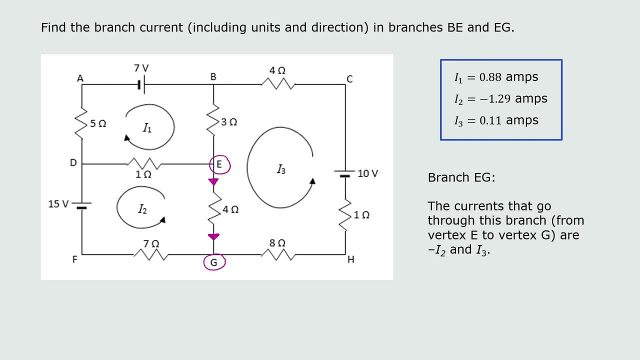 So I2 would be going up the branch from G to E. I3 would be going down the branch from E to G. So since we're looking from E to G, I3 is positive and I2 is negative. So the branch current in EG is negative: I2 plus I3,.